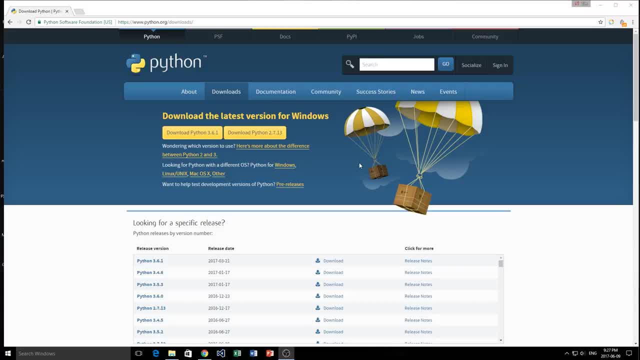 I recommend that you follow along with everything I'm doing in the tutorial. Pause the video at certain points, Rewind if you don't understand. It's important you understand these parts so that we can move forward into more complex ideas. So obviously the first thing that we're going to have to do if we're going to learn Python is we have to install it on our computer. So we're just going to go to the Python website up here. pythonorg slash downloads right here And all you're going to do is just click download Python 3.6.1. 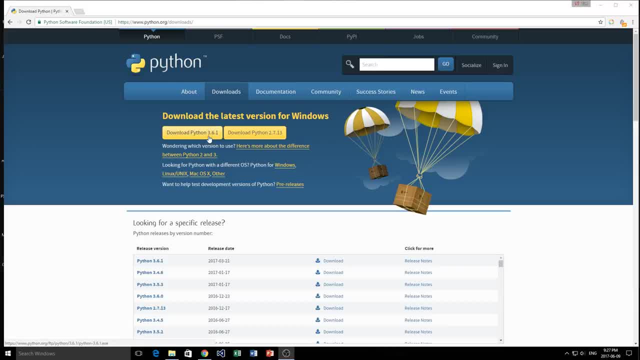 Now, I'm not going to do that because I already have Python installed and downloaded on my computer. But pretty much once you download this, it's going to pop up down here in your downloads folder. Just run the exe. It's very simple And you'll be running Python in no time. So now pause the video, Go ahead and do that, And then we can go to the next steps. 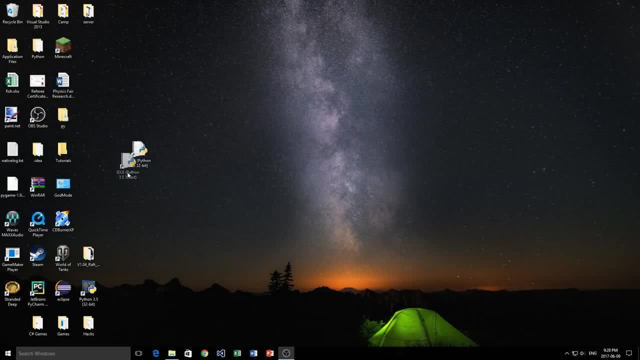 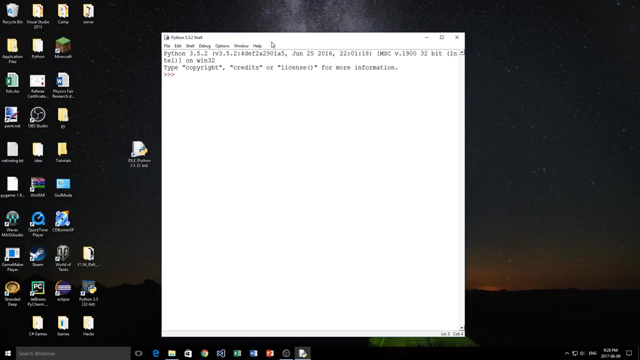 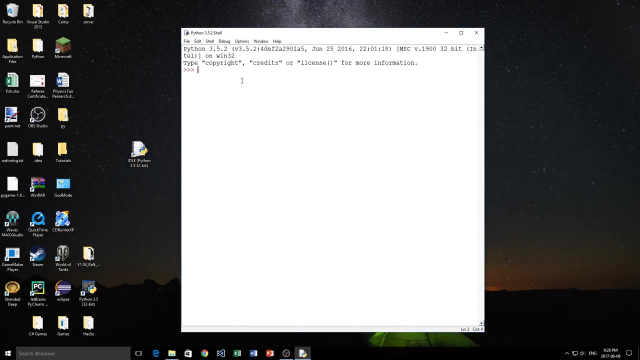 Okay. so once you've done that, you're going to notice that you have an application that looks like this. It's called IDLE Python, and then it'll have the version 3.5.. Don't worry if you have a version that is larger than that, So 3.6, or even one that's before that. Most of the things that I do in this will work in all the versions of Python. Okay, so go ahead and run the IDLE. You'll notice the first thing that pops up is the Python shell, As you can see at the top here. the shell- Now, this right here is not where we're going to write all our programs, It's the console kind of. So here I can type any lines of code. 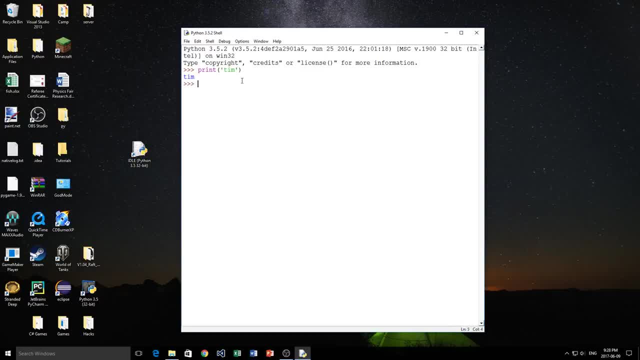 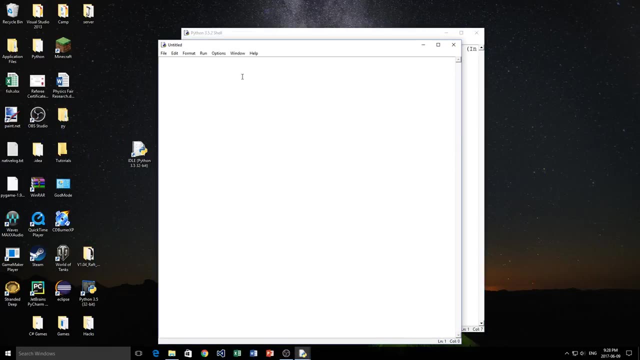 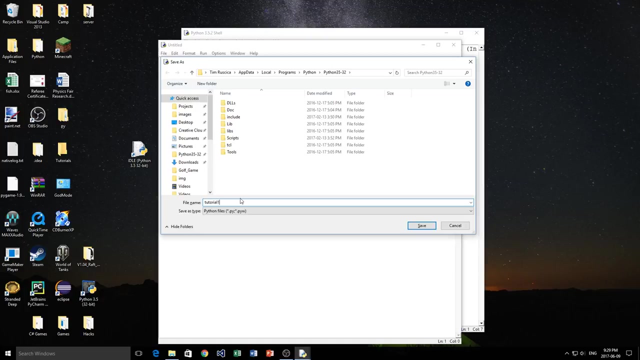 I want to print a name like this and it'll run right away. So that's not what we're going to do. You can play around with this if you want, but we're going to go to file and we're going to click new file, And then here we go. So now we have a new document that we're going to be working on and we're going to be programming it, So I'm going to go ahead and I'm going to save this right away as tutorial one into my tutorial folder, which I believe is on my desktop. 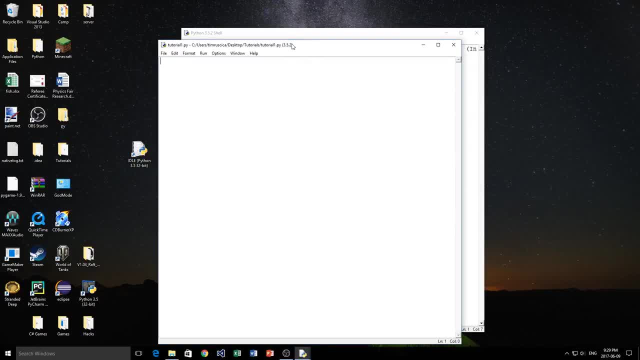 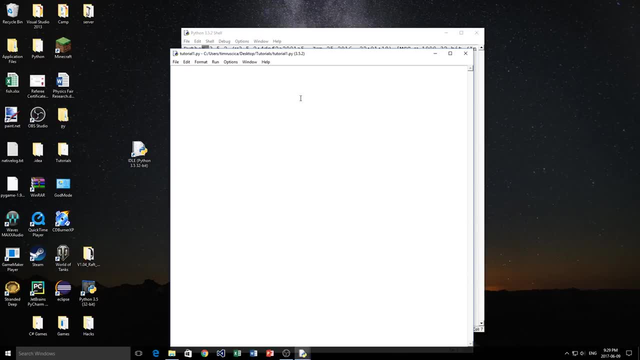 Right here, Yep, right there, Awesome. Okay, so there we go, We've saved it and now we're ready to learn a little bit about data types. So, pretty much, Python is a fairly basic language in comparison to a lot of other ones. A lot of things that it does is more simple than other languages, but it is important to understand the basic data types. So there's four main data types in Python. There is a few more, but we're just going to talk about these ones right now. The first one is an integer, So that can be a 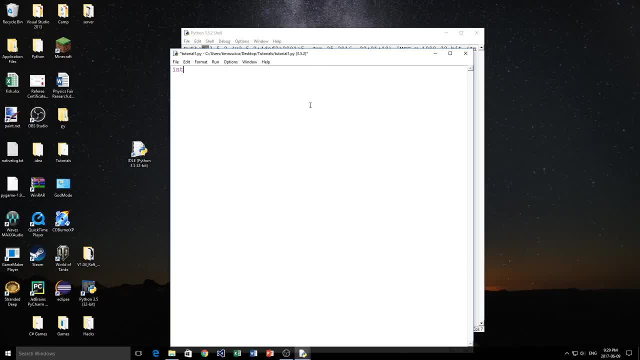 short form int. That stands for integer. Now, an integer is any number, So such as 1,, 4,, 76, any whole number. It's important that it is a whole number. It could be a negative number as well, negative 5, 0.. Those are all integers. Okay, now we have strings. Now, the short form for strings is str. Now, pretty much a string is anything embedded in quotations, So like this: this is my name Tim. 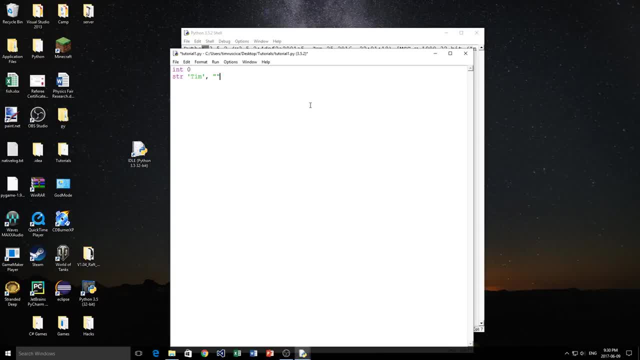 That is a string. And then we also have something like this: This would be a string. And even like this: this would be a string. So although there is a number in here, since it is between these two quotations here, it is a string. So even if I did another number like that string Now, it's also important to understand that it doesn't matter if you use the single quotations or the double quotations. Sometimes we use the single quotations. 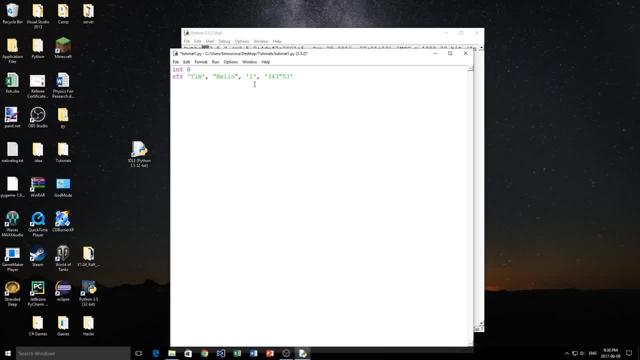 Because inside of our actual quotations we want to use double quotations, or maybe, if we use the double quotations, because we want to use the single quotations inside of our actual string, like that. Okay, so those are just a few examples. Now we have Boolean variables or data types. sorry So, Boolean data types is something like true and false. So true and false- pretty basic. 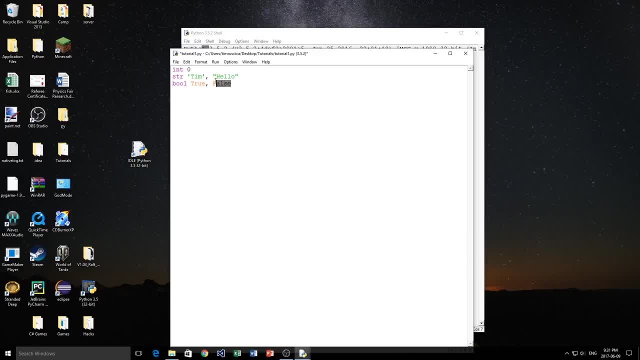 These are reserved words in Python, meaning that they're highlighted in yellow and that you cannot use them for variable names. That's going to be important later on. Just know that they are important words, true and false, and they do start with capitals. So, for example, if I type true like this, it's not highlighting orange right. So that's because true. in Python the keyword for that starts with a capital. So true and false. 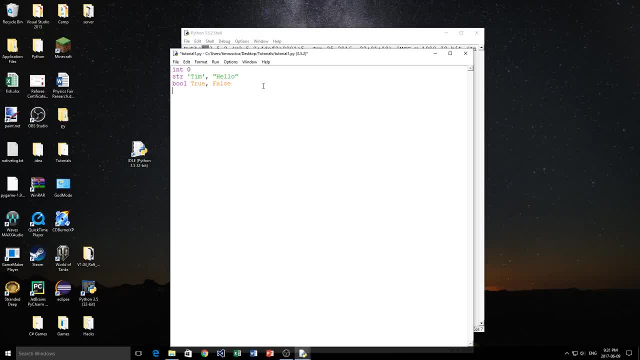 Then we have the decimal. So we have the decimals, which are the float data type, like this: So anything with a decimal floating point, so 1.23, anything like that- any decimal number with a floating decimal point would be a float. Okay, so those are the four basic data types. There is a few more that I'll go on to later on, but you just have to understand these ones right now. So, now that we know these data types, I'll give a quick little quiz here. 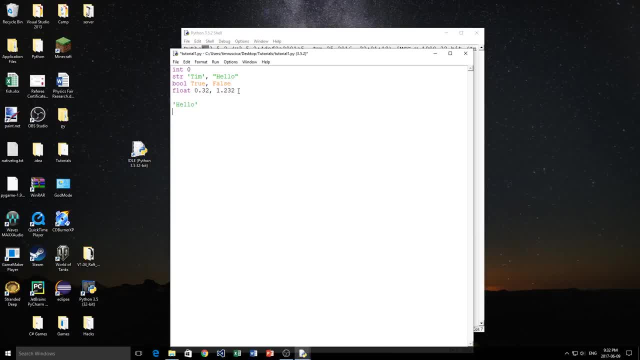 So I'm going to give a quick little quiz here. So I'm going to give a quick little quiz here, So I'm just going to put a few things right here and then I want you to pause the video and go ahead and try to determine what type of data type these things are. Okay, so go ahead, pause the video and then I'll go over the answers in a second. Okay, so we'll start with the first one here. hello, It's the same example that I have up here, except in single quotations, so we can see that it is a single quotation. 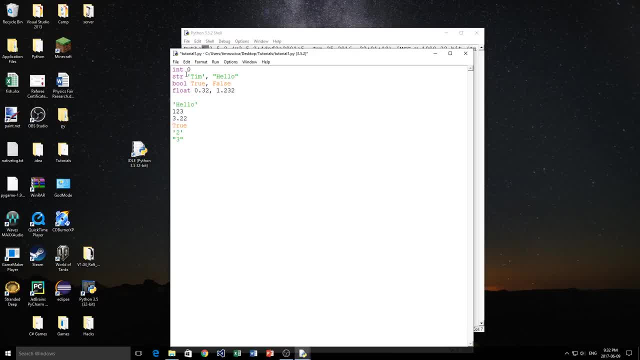 Okay, so that is a string data type. Okay, so that is a short form str. Now we have the number 123. That would be the integer data type. We have another number here that has a decimal point, so 3.22.. That would be a float. We have the keyword true. This data type is a Boolean data type. Then we have two in quotations. This is very important. We don't want to get this mixed up. This is a string. Some people may think that it's an integer. 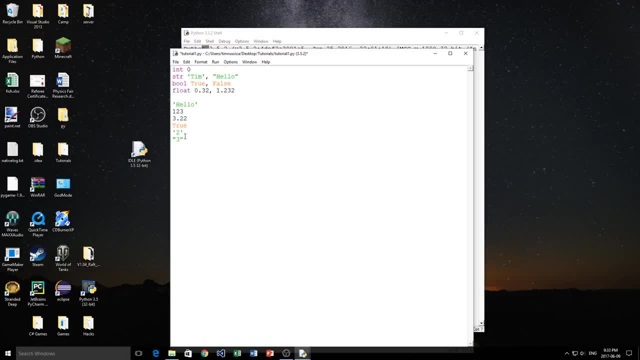 Because it's two. but no, it actually is a string because it is inside of the quotations. And then same thing here: three, inside of the double quotations. again is a string and not an integer. Okay, so now that we have an idea of the basic data types, I'm going to show you how to create a variable. So pretty much you may have heard of variables before in math or something like that. In math we tend to use x as a variable. We say x may be five, x may be four, anything like that. 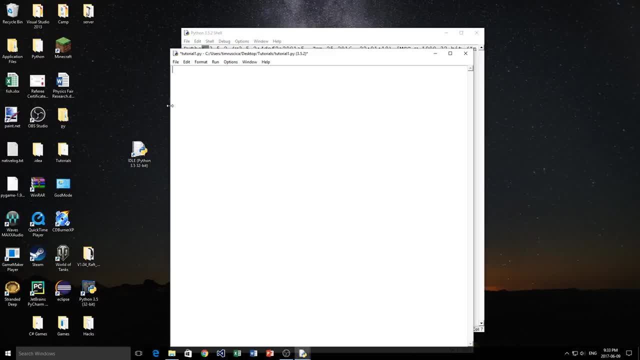 It's the same thing in Python. Now, declaring a variable in Python is very easy. All you have to do is type the variable name. So in this case, I'm going to use name and then simply give it a value. So this value, as you may remember, is a string. This is my name and I'm just storing it in the variable name. Now, if I want to access that variable, I want to see what that variable is. I can print it to the console by simply typing the variable name, which is name. So now we'll see what happens. 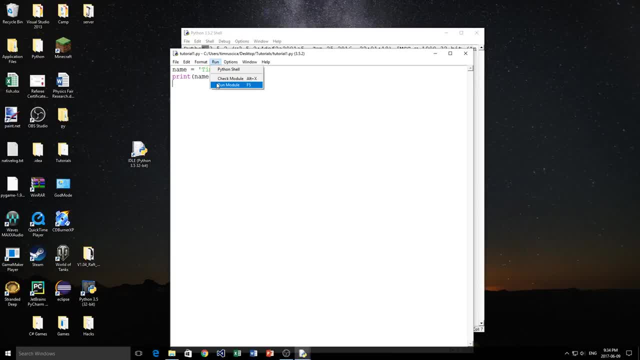 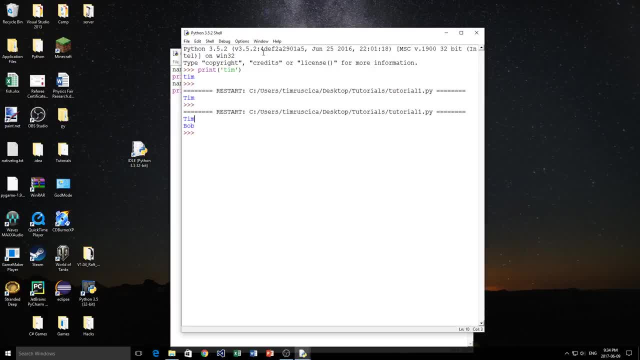 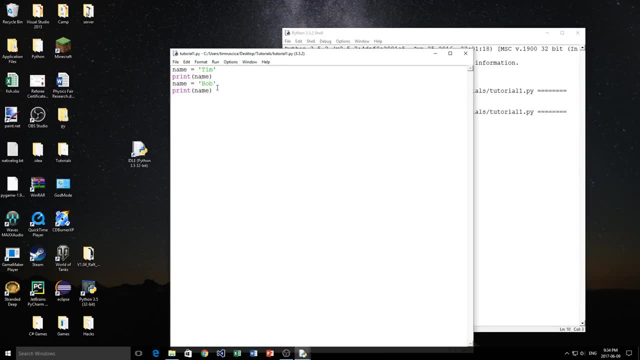 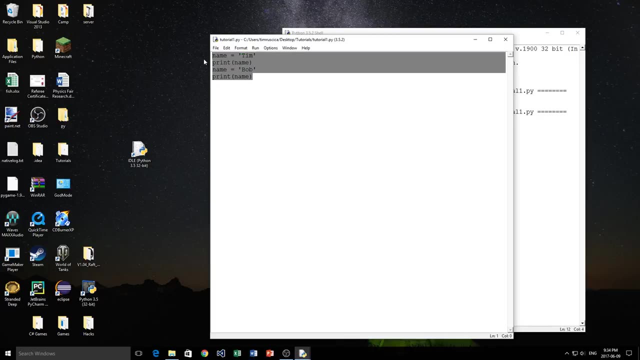 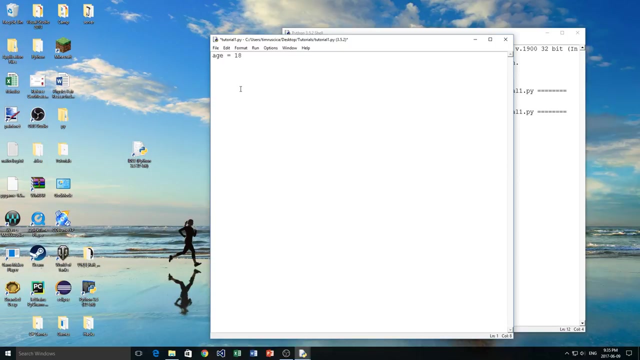 And then we'll see name, or, sorry, Tim and then Bob, So like we have here, name equals Tim, print name, name equals Bob, print name, right? So you've set it like that, Okay, so that's pretty basic. Now you can create variables of different data types. So, for example, if we had a variable age, I would use an integer data type, So like 18, for that variable, And then again, if I wanted to print it to the screen, I would type print And then 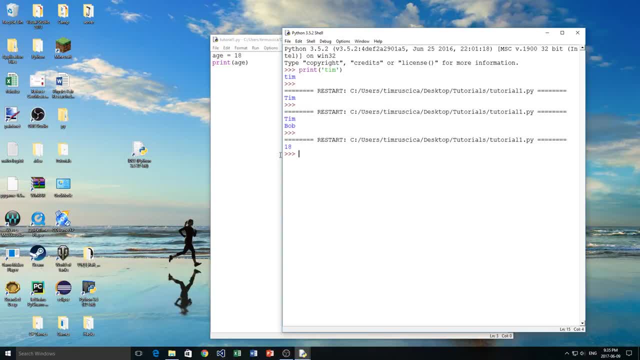 the variable name like that: Okay, 18.. Perfect, right. So we printed that to the screen. Again, if the variable names, there's a few restrictions on variable names. So here you just see I've used three lowercase letters. your variable names can contain underscores, they cannot contain dashes. they can only contain underscores text and they cannot start with a number. I believe So if I try to do.